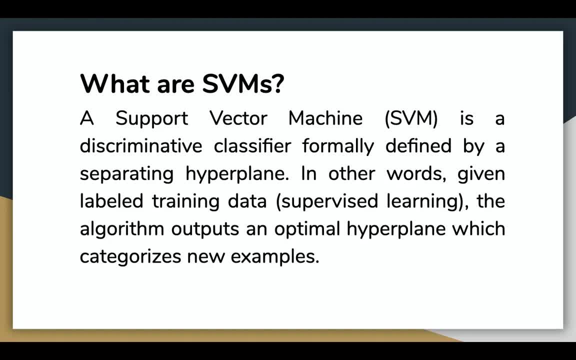 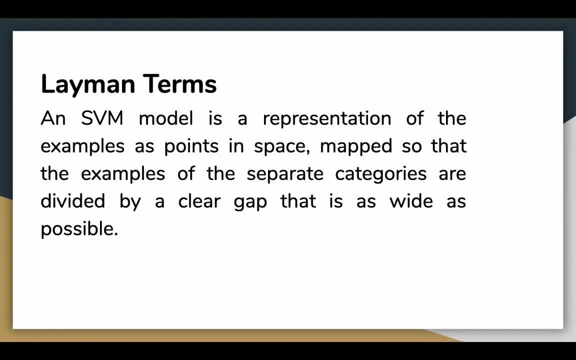 In other words, given labeled training data, the algorithm outputs an optimal hyperplane which categorizes new examples In simple terms. an SVM model is a representation of the examples as points in space mapped so that the examples of the separate categories are not separated. 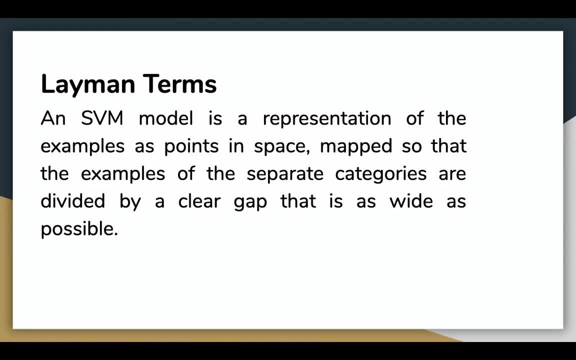 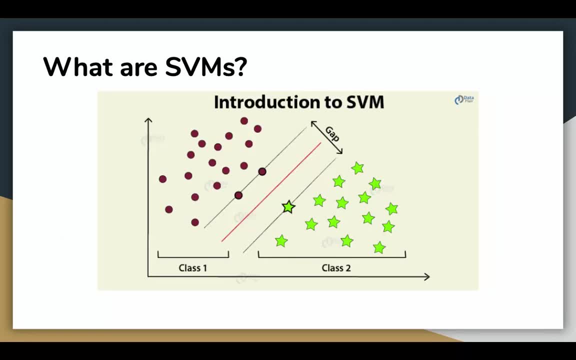 In other words, the examples of the separate categories are divided by a clear gap that is as wide as possible. Let's visualize this In this graph. we can see that the two classes are separated by the largest gap possible. The space between the red line and the closest point to the red line is called a margin. 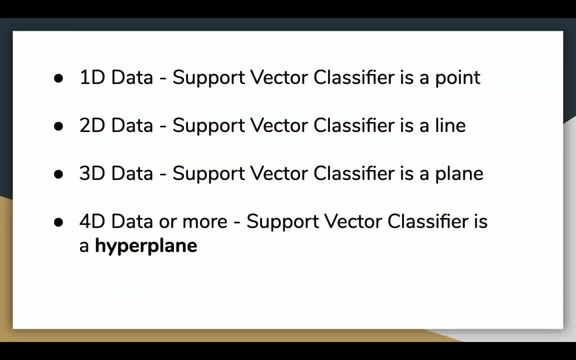 So, for one-dimensional data, the support vector classifier is a point. For two-dimensional data, the support vector classifier is a line, as seen in the previous slide. For three-dimensional data, the support vector classifier is a point. For three-dimensional data, the support vector classifier is a line. 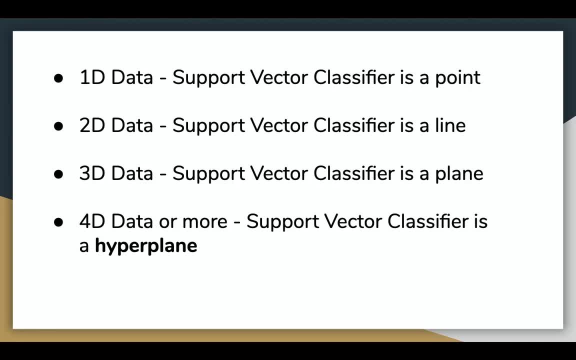 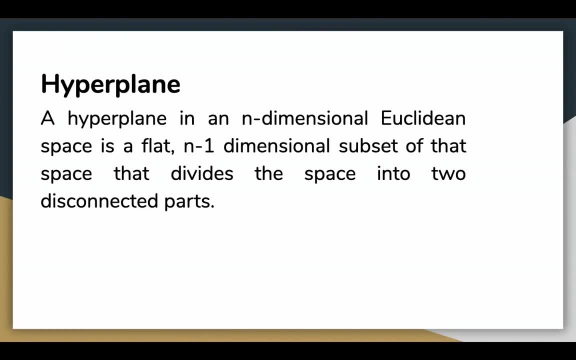 For four-dimensional data, the support vector classifier is a plane, And for four-dimensional or more, the support vector classifier is a hyperplane. So let's talk about the hyperplane now. A hyperplane in an n-dimensional Euclidean space is a flat n-1 dimensional subset of that space that divides the space into two disconnected parts. 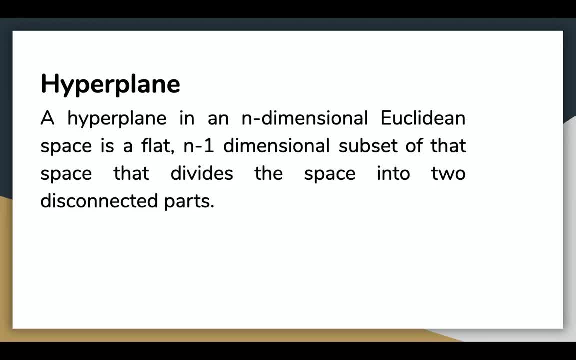 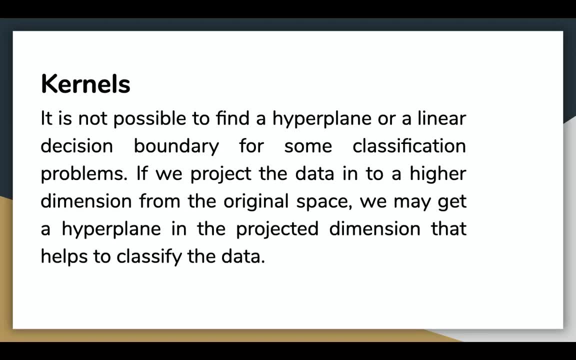 So a line is a hyperplane, or even a 2D plane for a 3D data is a hyperplane. SVM algorithm is a vector classifier. SVM algorithms use a set of mathematical functions that are defined as the kernel. Sometimes it is not possible to find a hyperplane or a linear decision boundary. 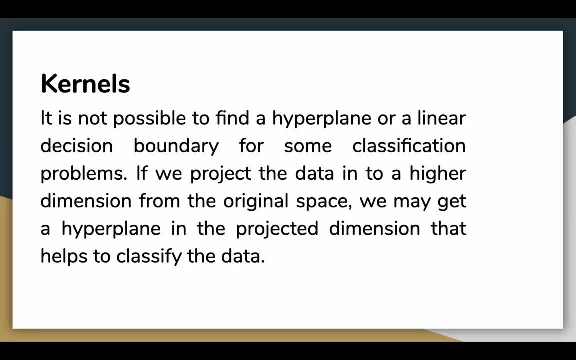 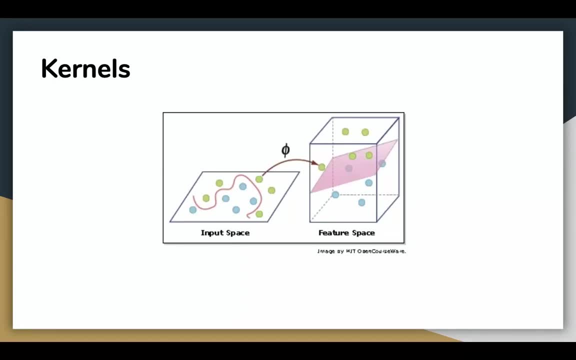 for some classification problems. If we project the data into a higher dimension from the original space, we may get a hyperplane in the projected dimension that helps to classify the data. Let's see what we mean here. As shown in the figure, it is impossible to find a line to separate the two classes, green and blue. 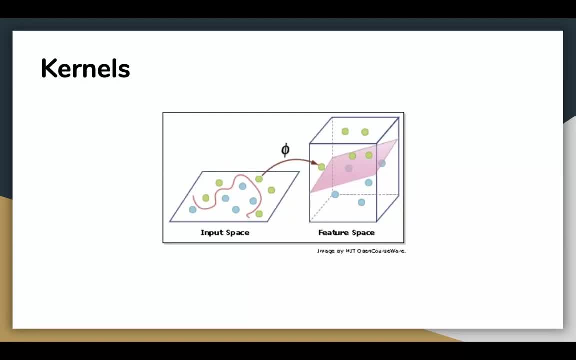 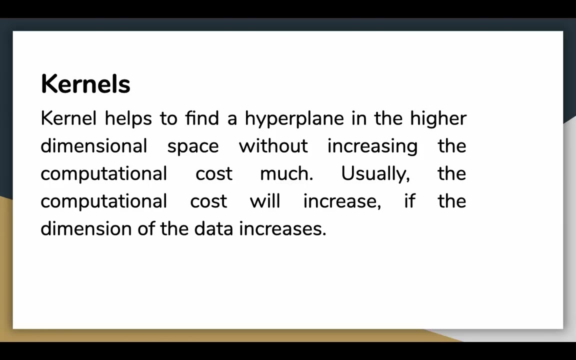 in the input space, But after projecting the data into a higher dimension we were able to classify the data using a hyperplane. Hence kernel helps to find a hyperplane in the higher dimension space without increasing the computational cost much. Usually the computational cost will increase if the dimension of the data increases. 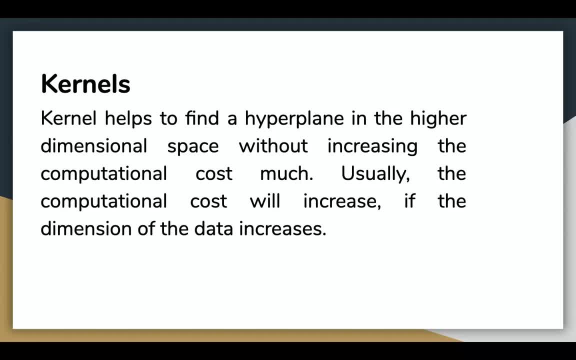 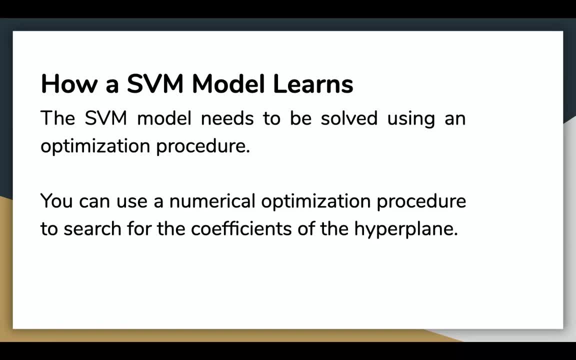 The mathematics behind how kernels work is out of scope for this video. The SVM model needs to be solved using an optimization procedure. You can use a numerical optimization procedure to search for the coefficients of the hyperplane. The most popular method for fitting an SVM is the sequential minimal optimization. 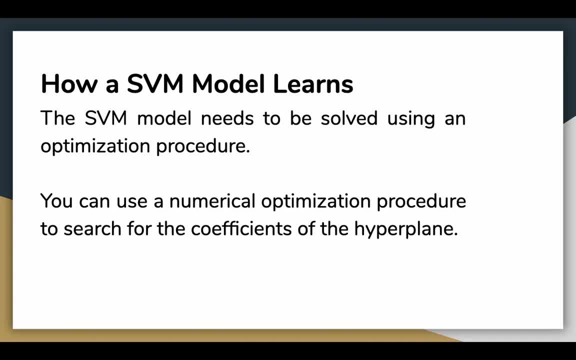 method that is very efficient. It bakes the problem into subproblems that can be solved analytically, by calculating, rather than numerically, by searching or optimizing. In the next video, we'll look at how to solve an SVM problem using a hyperplane. 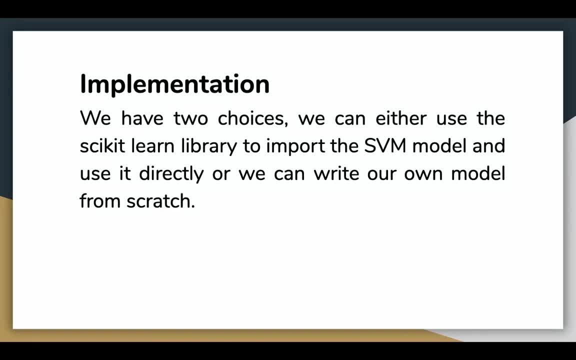 In the next video we'll implement a support vector machine. We have two choices here. We can either use the scikit-learn library to import the SVM model and use it directly, or we can write our own model based on the equations above. 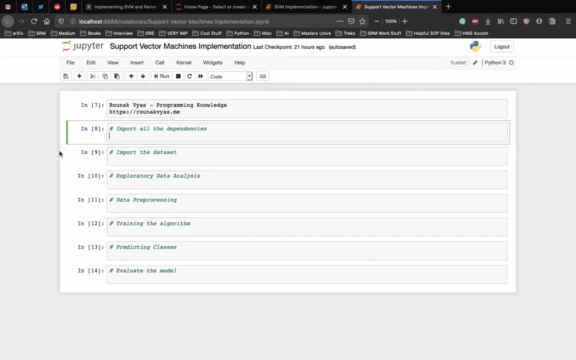 We'll talk about implementing support vector machines. A support vector machine is a type of supervised machine learning classification algorithm. SVMs were introduced initially in the 1960s and were later refined in the 1990s. However, it is only now that they are becoming a part of the machine learning class. 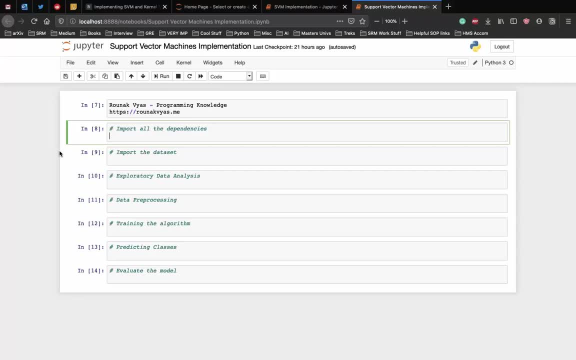 SVMs are becoming extremely popular owing to their ability to achieve brilliant results. SVMs are implemented in a unique way when compared to other machine learning algorithms. In this video, we'll implement support vector machines with the help of the scikit-learn library. 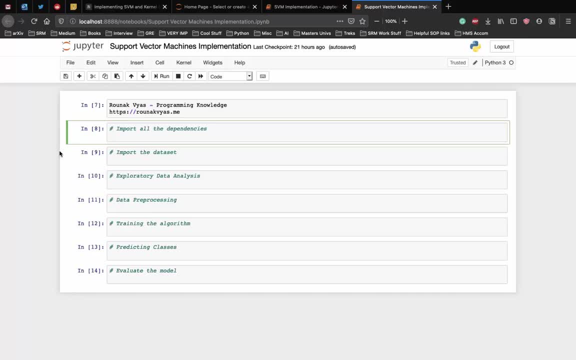 For the implementation. our task is to predict whether a bank currency note is authentic or not, based on four attributes of the note. Those attributes are the skewness of the wavelet performed image, the variance of the image, entropy of the image and the kurtosis of the image. 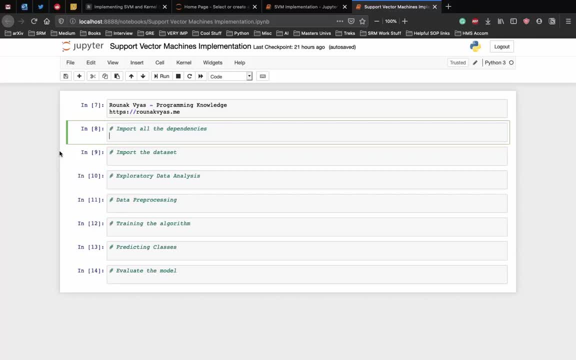 This is a binary classification problem and we will use the SVM algorithm to solve this problem. The detailed information about the data and a link to download the dataset can be found in the description. Download the dataset and store it locally on a computer where you intend to write the. 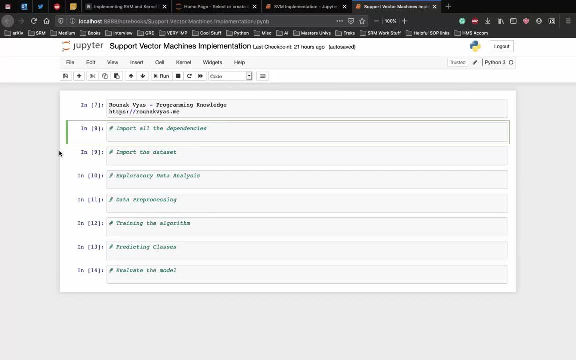 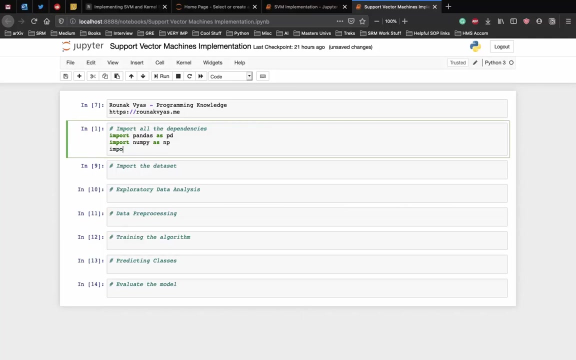 implementation. So let's start the implementation by importing all the necessary libraries. First we need to import pandas, as we need to store our data in a data frame, And the next is numpy, followed by matplotlib, and then we need the scikit-learn modules. 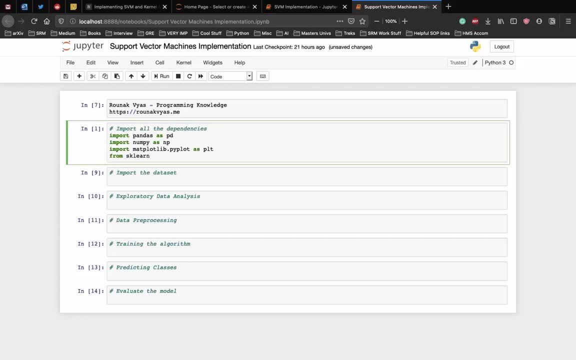 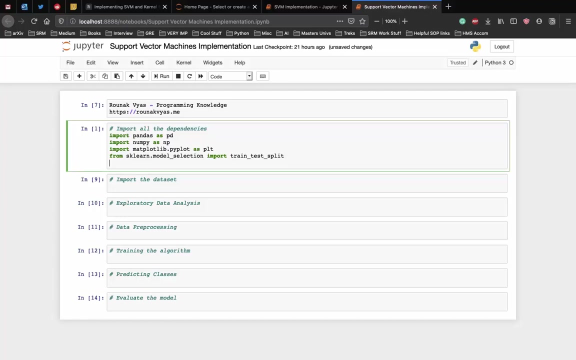 context. Here we'll be using train-test-split module, which we had not in the previous video for linear and logic regression implementations, But for SVM we'll have a train-test-split within SVM and see how the algorithm works on test data. next we need to import the SVM class. 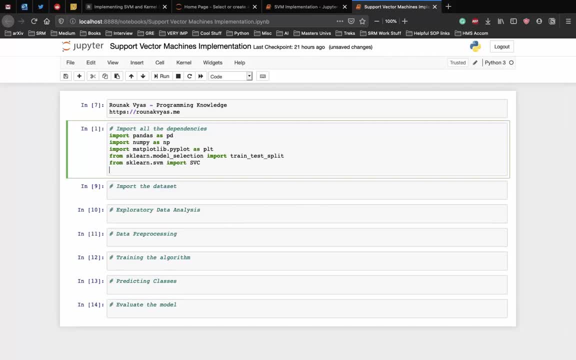 this SVC support vector classifier and at last, we need to evaluate our algorithm, so we'll need some metrics for that, and let's use the classification report module and, yeah, I think we're done so. now let's import the data. okay, I think we have some problem. yeah, it's a. 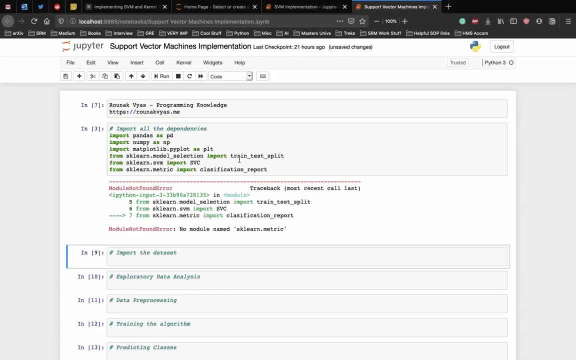 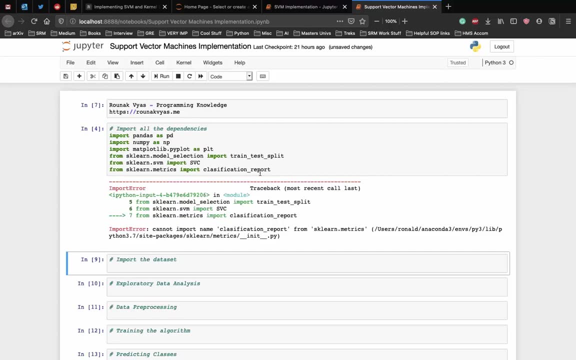 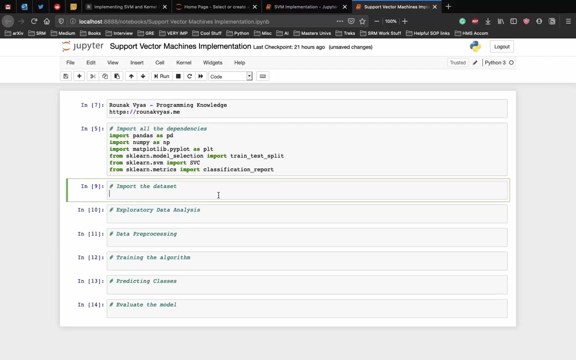 spelling mistake. metrics have a lot of spelling mistakes here. okay, now let's import the data into a program. to read the data from the CSV file, the simplest way is to use the read CSV method of the pandas library. the following code, which I'm going to write, is going to read the: 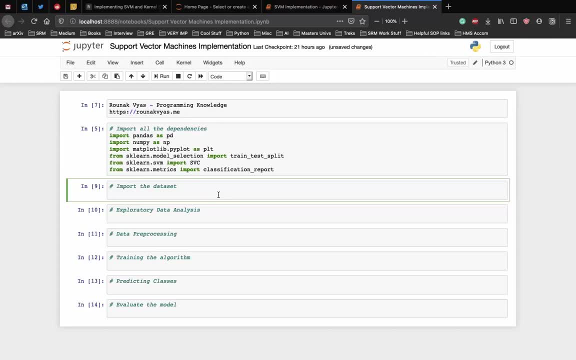 bank currency note data into a pandas data frame. let's have bank data equal to PD dot read CSV, and the name of the CSV file is bill authentication, which you can find in the description of the video. okay, now they are virtually limitless ways to analyze datasets with a variety 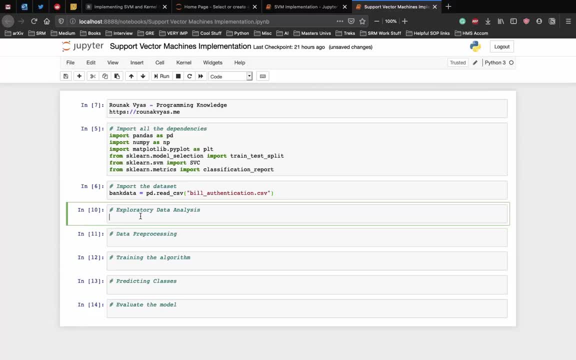 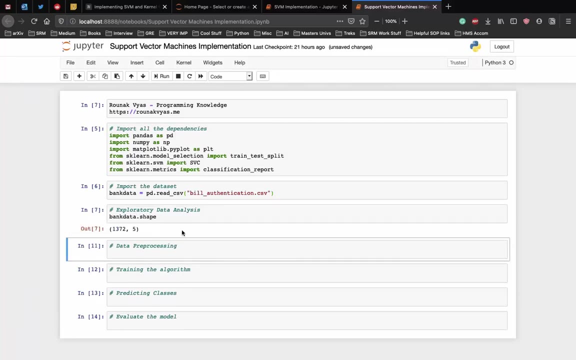 of Python libraries. for the sake of simplicity, we will only check the dimension of the data and see the first few rows. to see the rows and columns of the data, execute the following command and in the output you see one, three, seven two comma five. this means that the bank. 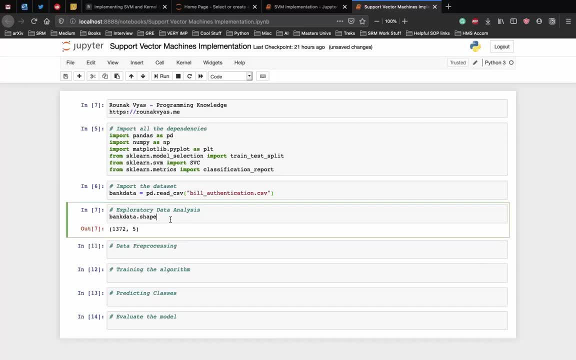 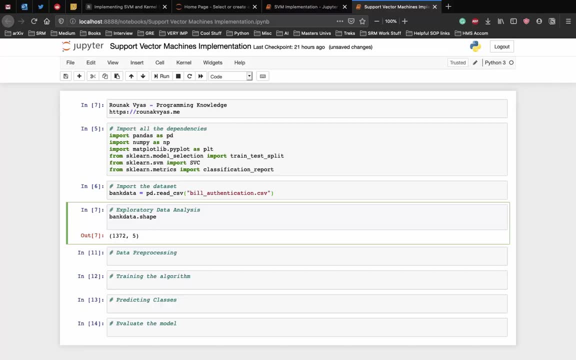 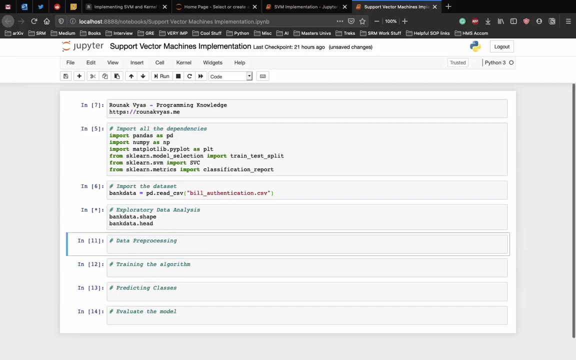 node data set has one, three, seven, two, 2 rows and 5 columns. Now to get a feel of how our dataset actually looks, let's actually see the first 5 rows of the dataset using the head command, And here you can see the. 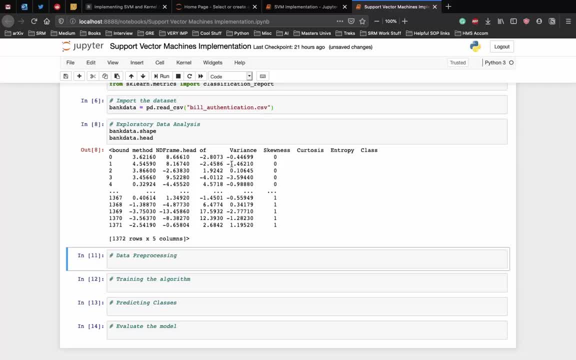 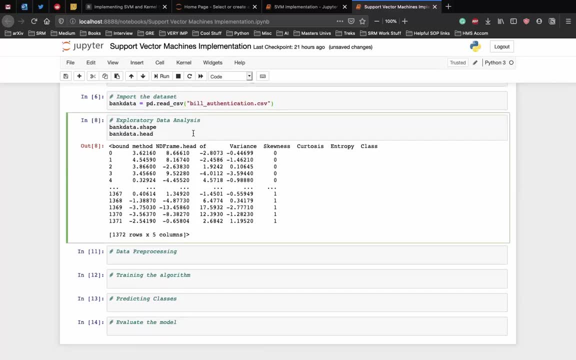 first 5 rows of dataset and you can also see. the attributes of the dataset are numeric. The label is also numeric, that is class 1 or 0.. Let's preprocess the data before training the model. Data preprocessing involves two steps. First, dividing the data into attributes. 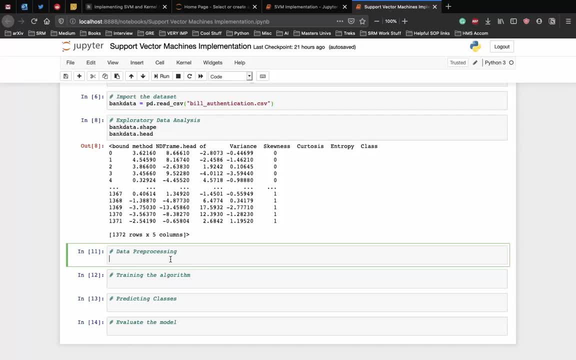 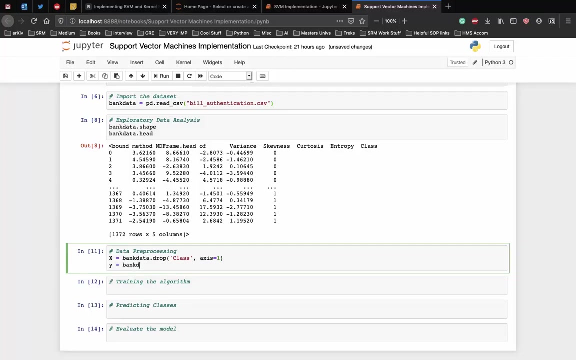 and labels. and second, dividing the data into training and testing sets. To divide the data into attributes and labels, execute the following code: Let x equal to the attributes, so bank data. In the first line of the script, in the cell, all the columns of the bank data dataframe. 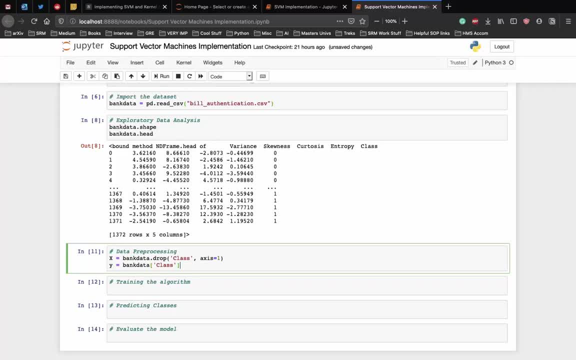 are being stored in x, except the class column, which is the label column. The drop method drops this column. In the second line. only the class column is being stored in the y variable. At this point of time, x variable contains attributes, while the y variable contains corresponding 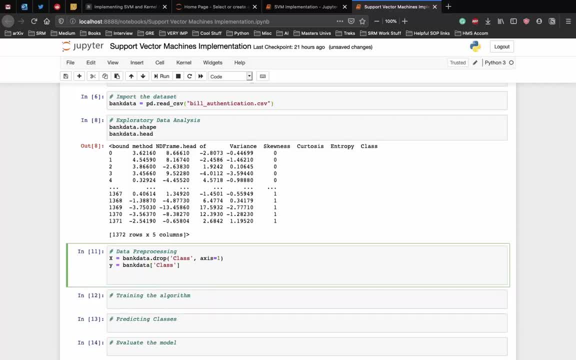 labels. Once the dataset is divided into attributes and labels, the final preprocessing step is to divide the data into training and test sets. Luckily, the model selection library of the scikit-learn library contains the train-test-split method that allows us to seamlessly divide the data into training and test sets. 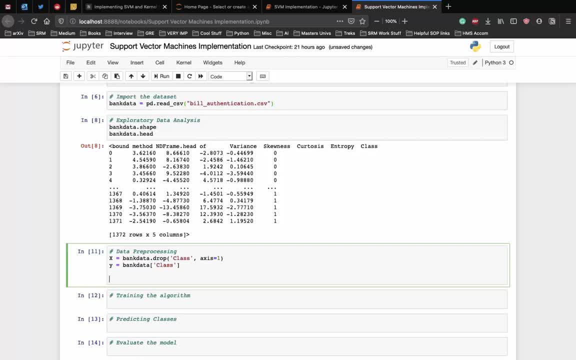 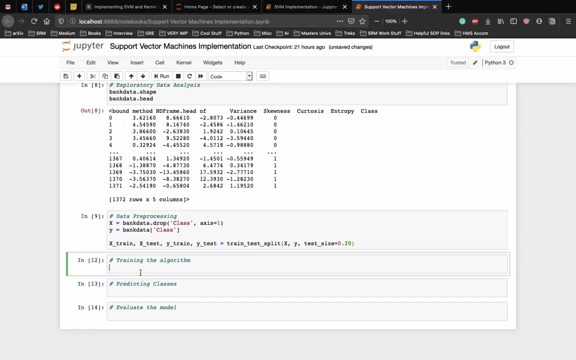 Let's write the code for that: x train, x test, y train, y test, train, test-split, and we want the test size to be 20%. We have divided the data into training and testing sets. Now is the time to train our SVM on the training data. 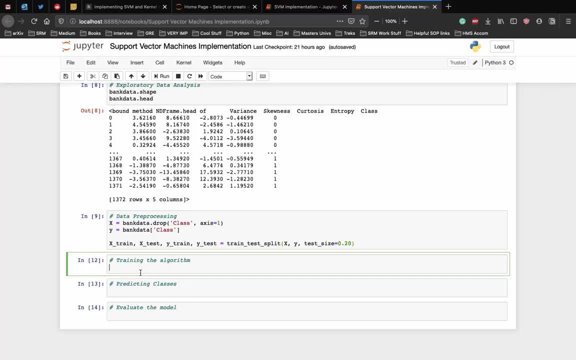 Scikit-learn contains the SVM library, which contains built-in classes for different SVM algorithms. Since we are going to perform a classification task, we will use the support vector classifier class, which is written as SVC in the Scikit-learn's SVM library. 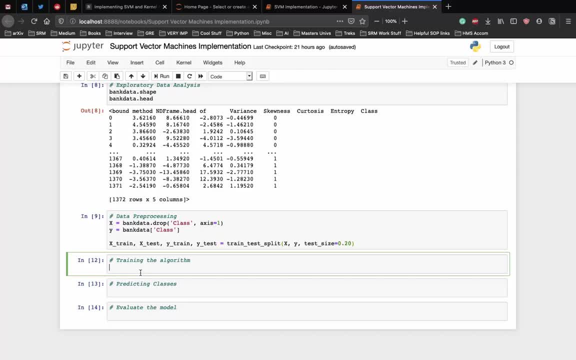 This class takes one parameter, which is the kernel type. This is very important. In the case of a simple SVM, we simply set this parameter as linear. since simple SVMs can only classify linearly separable data, Let's write the code for that. so SVC classifier is equal to SVC and the kernel is equal to. 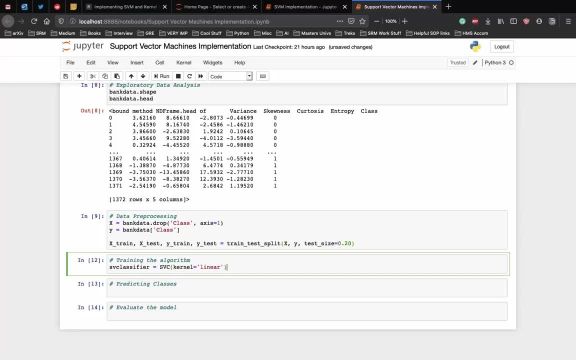 linear. The fit method of the SVC class is called to train the algorithm on the training data which is passed as a parameter to fit the fit method. svc classifierfit: xtrain, ytrain. To make this fit we will use the training method. 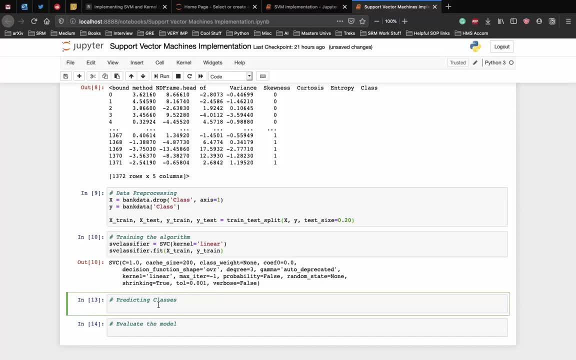 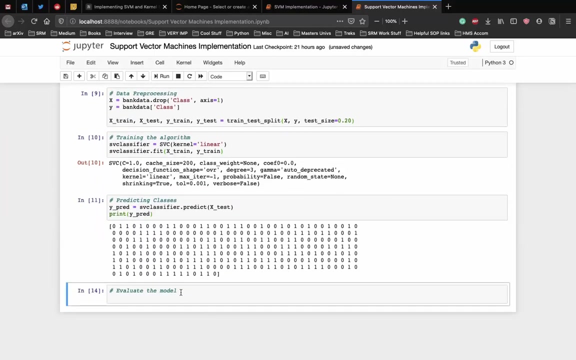 To make predictions, the predict method of the SVC class is used. yprediction is equal to svclassifierpredict- xtest and let's actually print ypred to see our predictions. As you can see, the algorithm has been run on the xtest data and all the predictions.